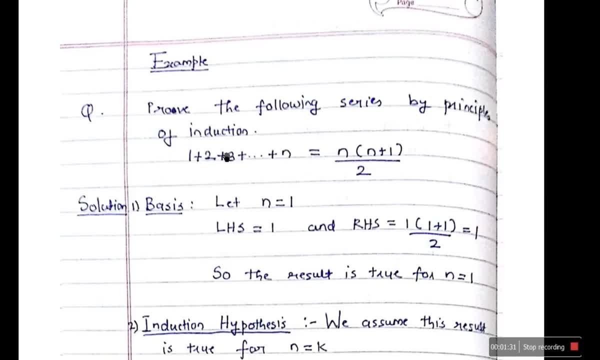 one prove that the following series of principles of induction- okay, by principle of induction. so what is the series given to us? one plus two plus three, plus dot, dot, dot, dot till n is equal to n into n plus one upon two. so we have to prove that this series is true. so first step is called: 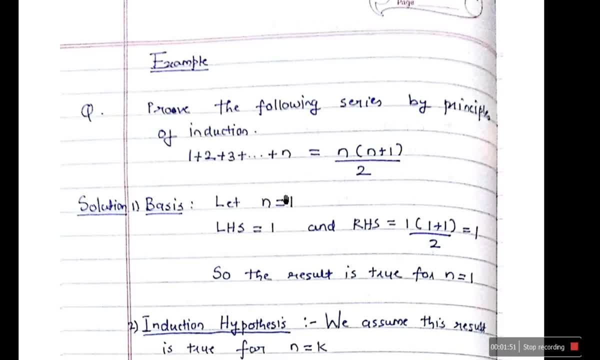 basis. yes, so where we take n equal to 1. now let's say we substitute the value of 1 over here. so 1 means only one value. so lhs it is only 1 and rhs will be 1. so you replace n with 1. 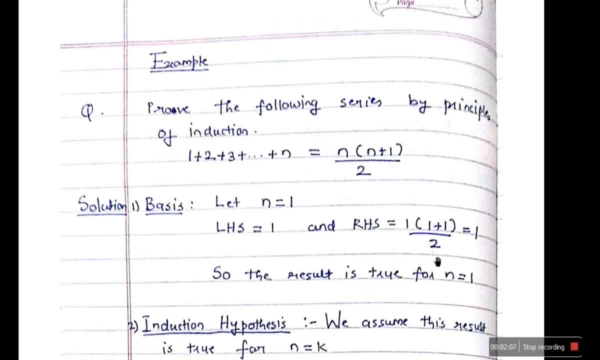 so you replace 1, so you will have a new value, n plus 1, which is equal to 1.. so it is true. so we have to prove that this series is true. so now the fourth step is hundred. so 1 into 1 plus 1 divided by 2, so that is 2 by 2, which is equal to 1. so lhs equal to rhs, proved. 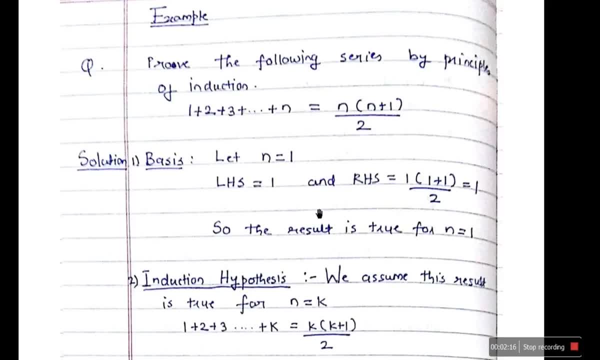 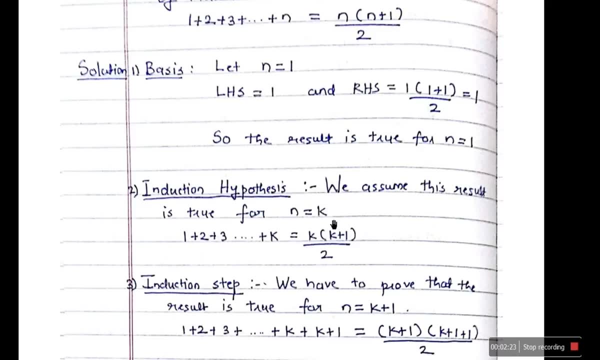 yes, so result is true for n equal to 1. first step is done. second step is induction hypothesis. now we assume that the result is true for n equal to k. that's why we just substitute instead of n, we substitute k. so we have 1 plus 2 plus 3 plus dot, dot, dot till k is equal to k into k plus 1 divided. 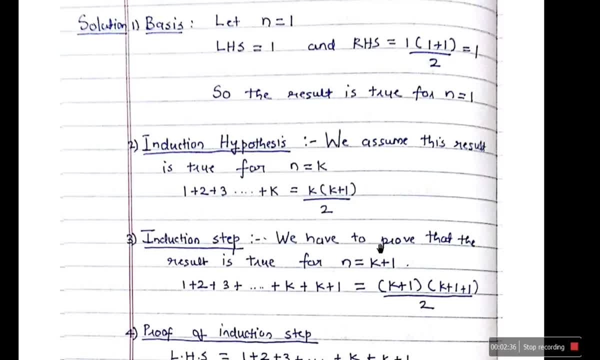 by 2. third step is induction step. okay, so over here, what we do is we prove that the result is true for n equal to k plus 1. so, again, what we have to do, we have to go for 1 plus 2 plus 3 plus 4. 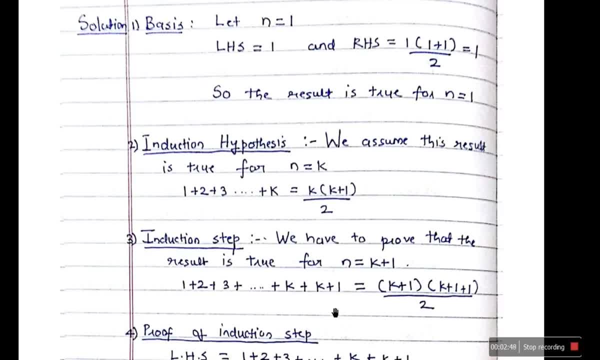 plus dot dot dot till k plus k plus 1. okay, what will be the answer? instead of k, you just replace it with k plus 1, so we get k plus 1 into k plus 1 plus 1. okay, divided by 2, so you are replacing. k plus 1 into k plus 1 plus 1. okay, divided by 2, so you are replacing k plus 1 into k plus 1. so you are replacing k plus 1 into k plus 1, into k plus 1. okay, divided by 2, so you are replacing. 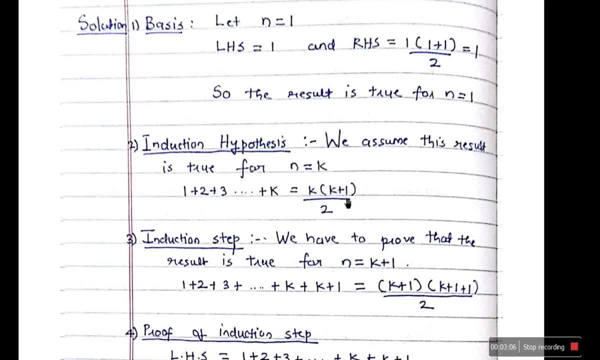 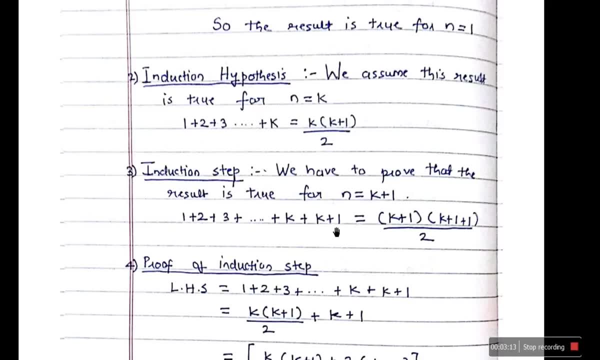 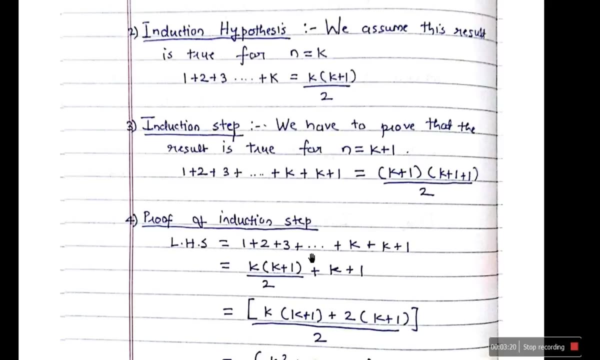 over here. instead of k, you're going one more step, so it will be k plus 1 plus 1. okay, now final step is: we have to prove that what statement we have made over here. that is induction step. we have to prove that it is true. now lhs is equal to 1 plus 2 plus 3 plus dot, dot, dot, dot plus k plus k plus.